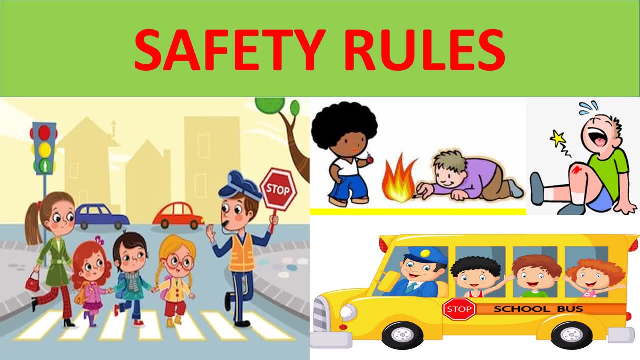 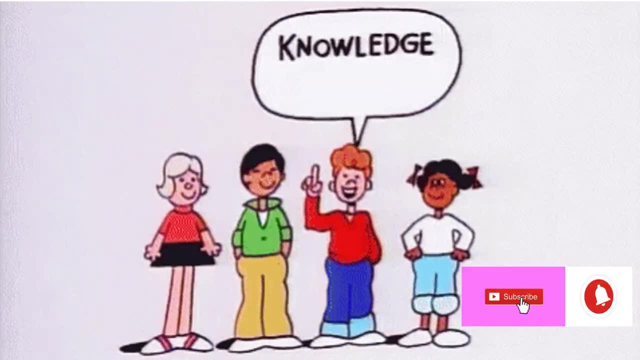 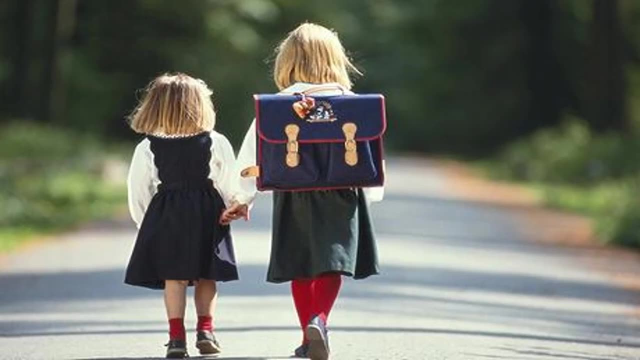 Safety Rules. Every day, you will be notified with a new video which improves your knowledge day by day, So don't forget to subscribe and click the notification bell. When we are at home or walking on the road or playing in the ground, we have to remember some safety rules. 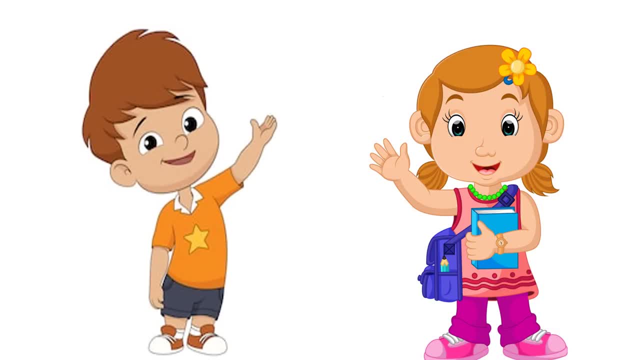 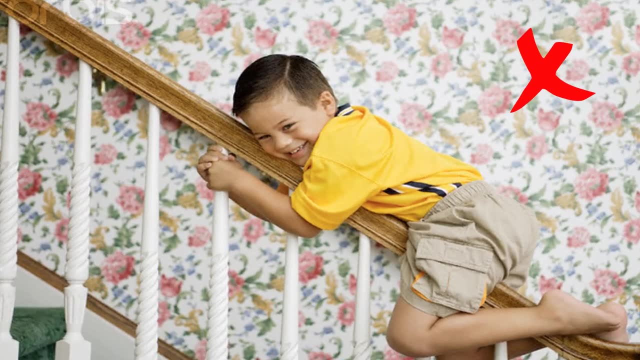 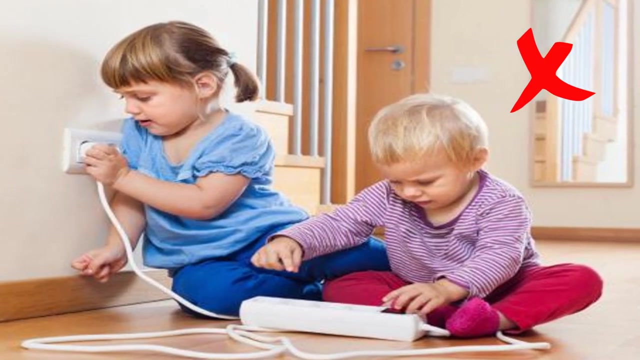 Safety rules protect us from harm. We must follow safety rules everywhere. Safety begins at home. Do not glide on the railing, Do not play on rooftops or an open balcony, Never touch electric wires. Never play with knives and blades. 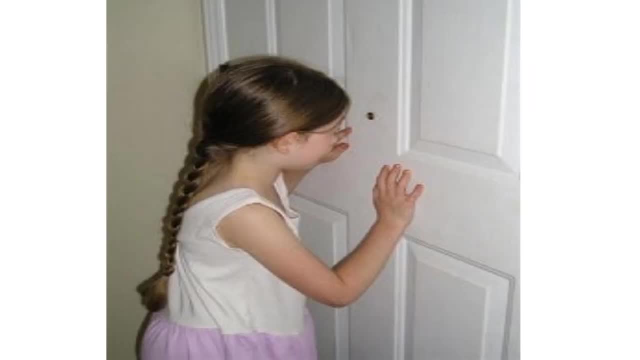 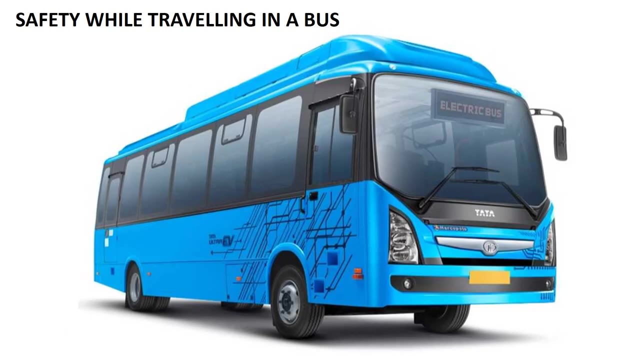 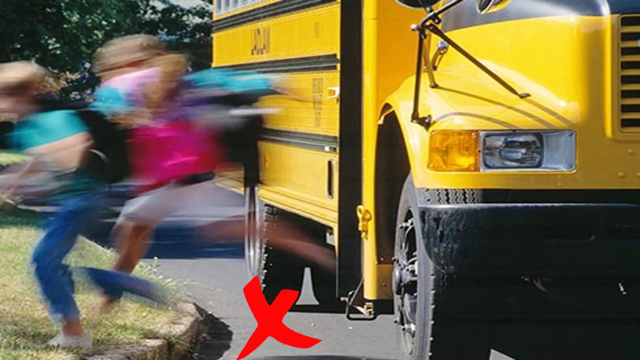 Never open the door to strangers. Never play with fire. Don't play with matchsticks. Safety while traveling in a bus. Stand in a queue at the bus stop. Do not get on or off a moving bus. Never talk to the driver while he is driving. 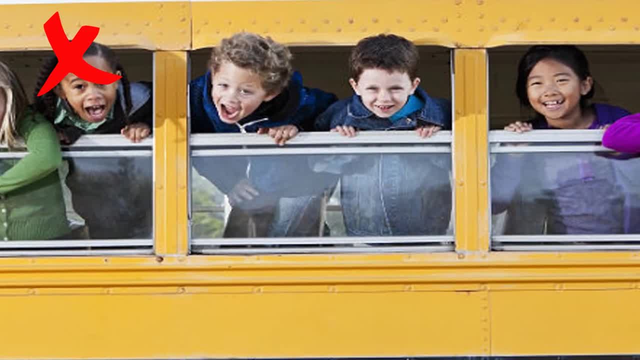 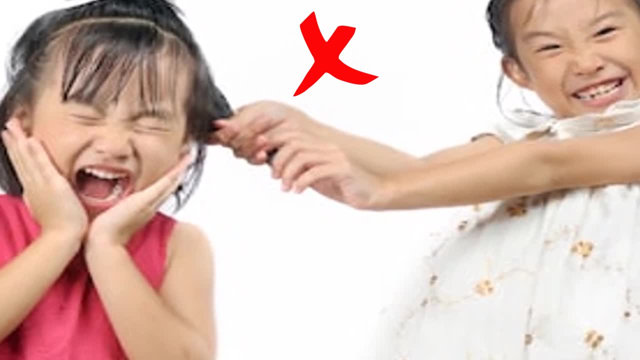 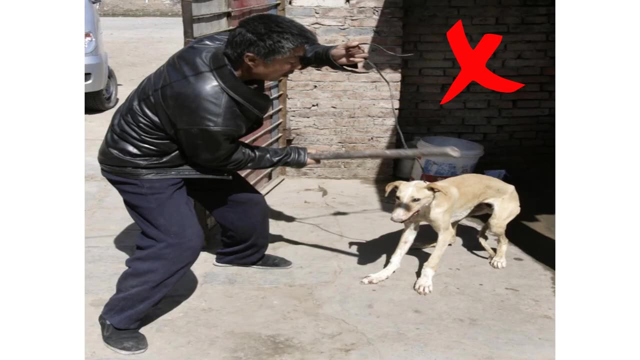 Do not lean out of the window of a bus. Safety while you play. Do not do any mischief while playing. Do not play near manholes. Never play in deep water or near fire. Do not tease animals. Safety on the road. 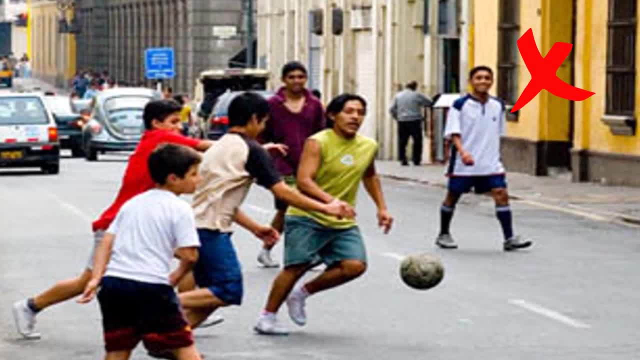 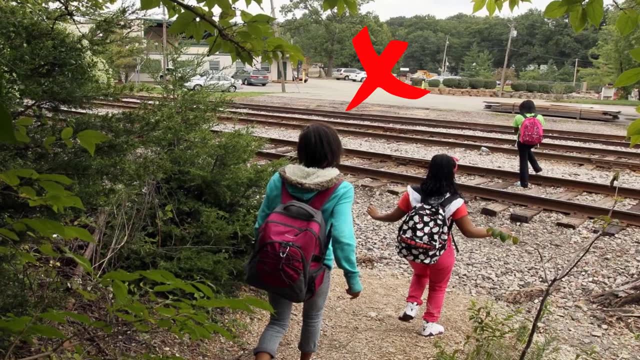 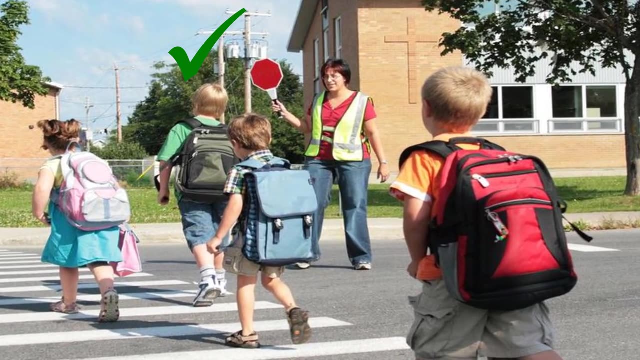 Never play on the road. Always walk on the footpath. Use the overhead bridge while crossing the railway line. Cross the road only at the zebra crossing Cross when there is no traffic. Before crossing the road, we must first look to our right, then look to our left and then right again. 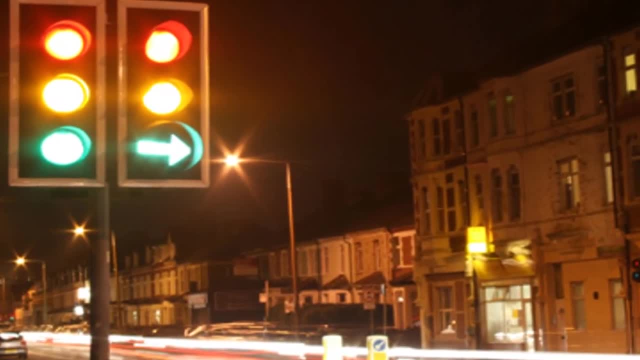 Cross when there is no traffic. Before crossing the road, we must first look to our right, then look to our left and then right again. We must obey traffic rules. Let us learn the traffic signals. Stop says the red light. 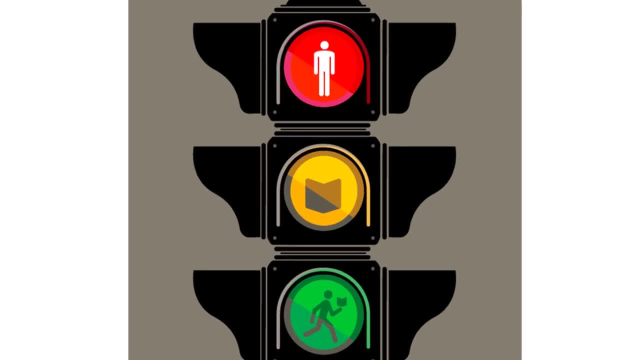 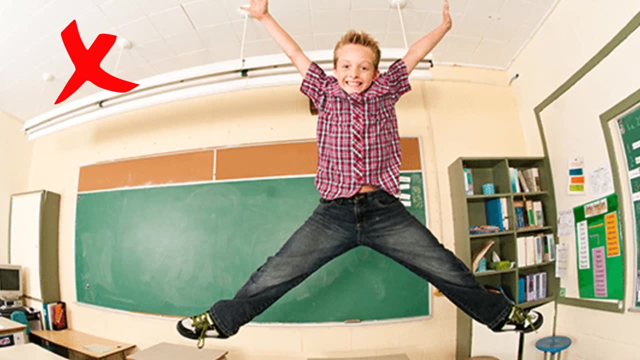 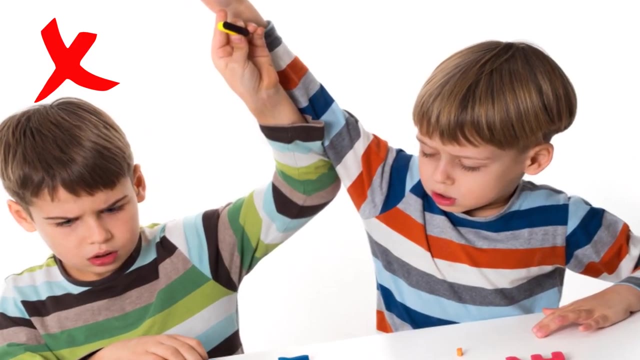 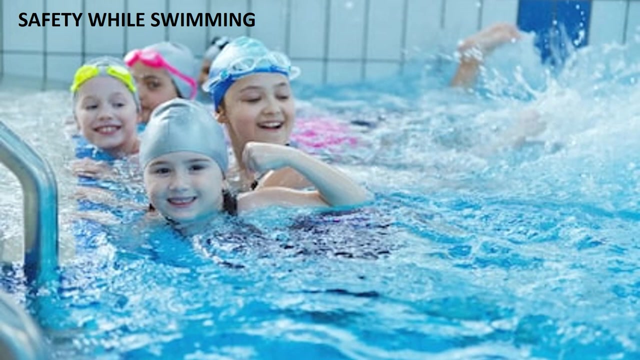 Wait, says the yellow light, Go, says the green light. Safety in the classroom. Do not jump over chairs and desks While in class. do not push and pull each other. Do not hit your classmates. Safety while swimming. 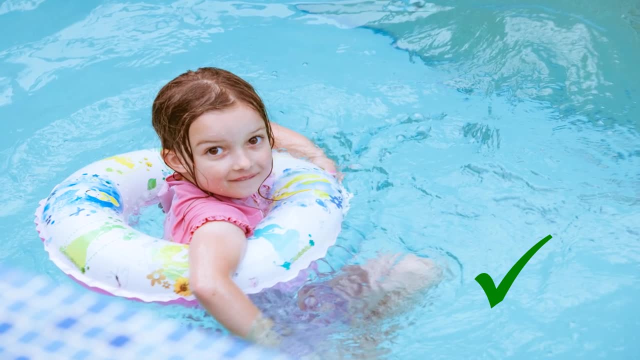 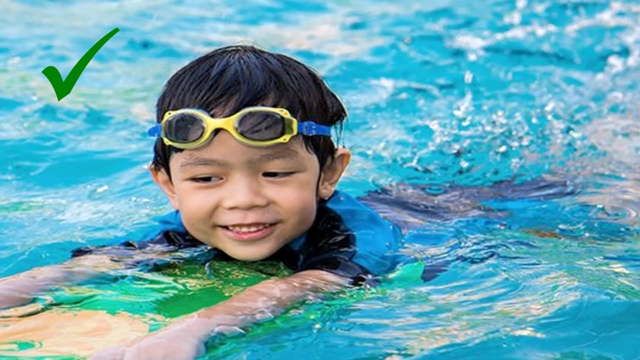 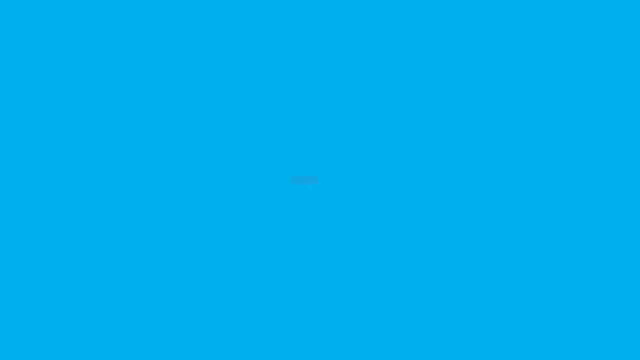 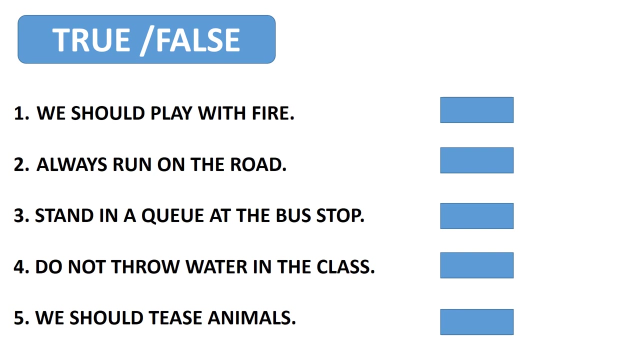 Always use a tire tube. if you are a learner, Always swim in the part of the pool which is not deep. Ask a grown-up person to be with you when you swim. Question time. Say true or false for the following: We should play with fire: Answer False. Next question. 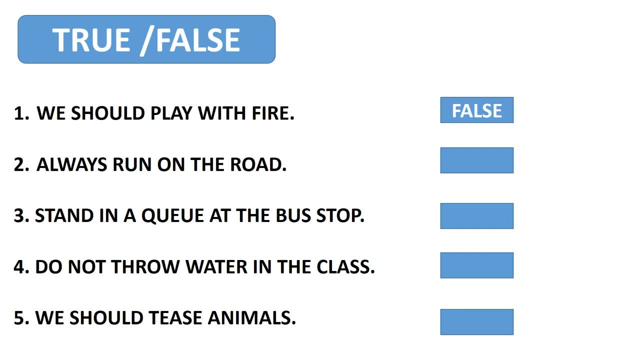 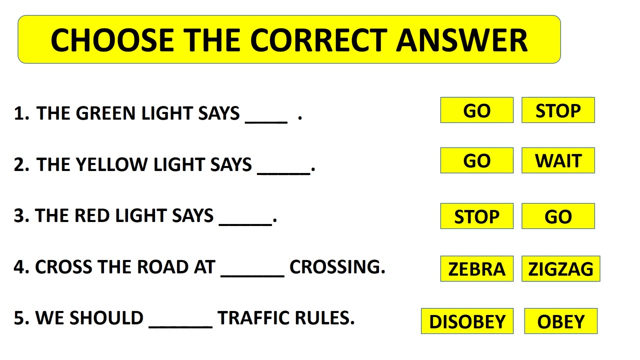 Always run on the road? Answer False. Next question: Stand in a queue at the bus stop. Answer True. Next question: Do not throw water in the class Answer- Answer True. Next question: We should tease animals. Answer False. Choose the correct answer. The green light says: Answer Go Next question. 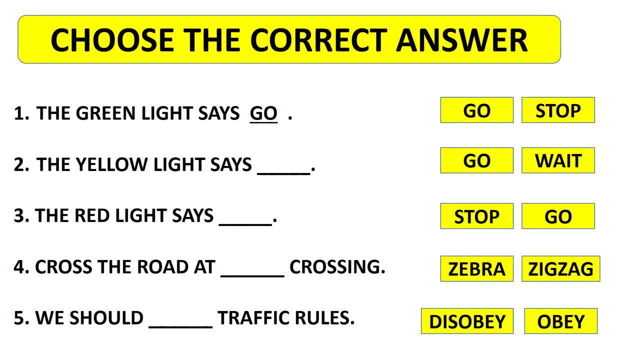 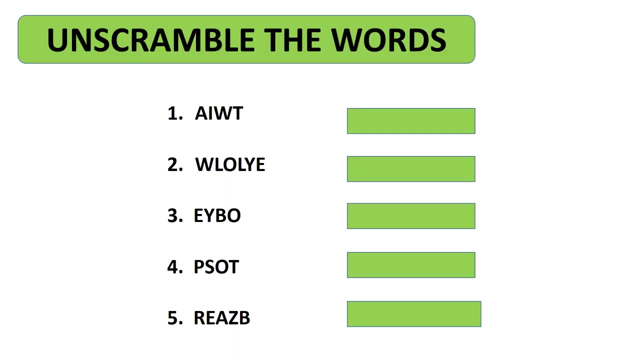 The yellow light says True. Answer: Wait. Next question. The red light says Answer. Stop. Next question: Cross the road at crossing. Answer: Zebra. Next question: We should traffic rules. Answer: False: obey, unscramble the words. you get 30 seconds to complete it. you match the following: